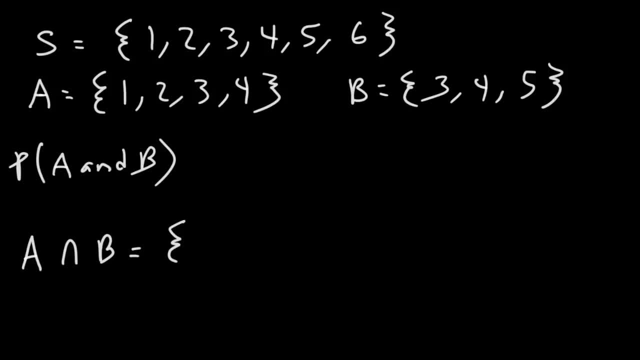 intersection of A and B. So the numbers that corresponds to event A and B are three and four. Now the probability is equal to the number of favorable outcomes divided by the total number of possible outcomes. So we have two numbers, where A and B will both be occurring, out of six potential outcomes. So the 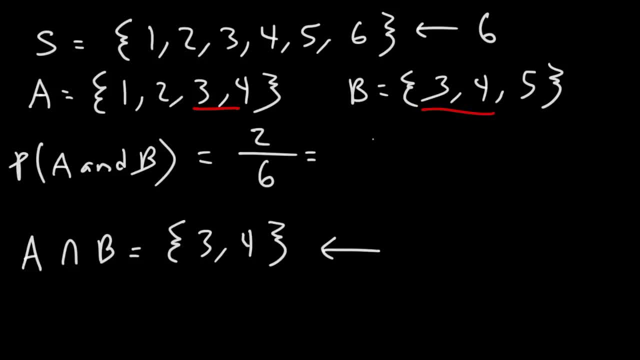 probability is going to be two over six, which we can reduce that Two is two times one, Six is three times two, And so this becomes a probability of one over three, which, as a decimal, that's 0.33 or 33%. That's the routed answer. Now what about the probability of event A or event B? 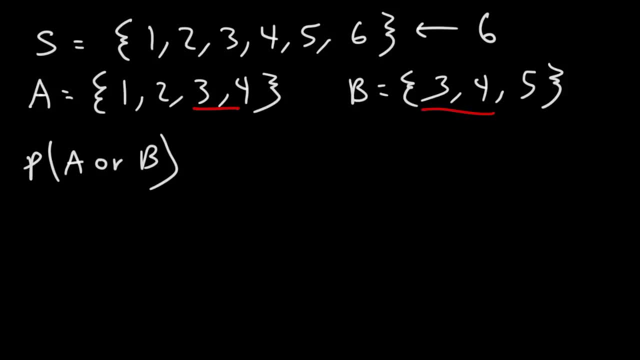 occurring. What's the answer to that question? Let's write the sample space of A or B. So this is going to be the union of these two events. So basically it's going to be all these numbers combined. Event A occurs anytime we get a one, two, three or four. B occurs if we get a three, four or five. So 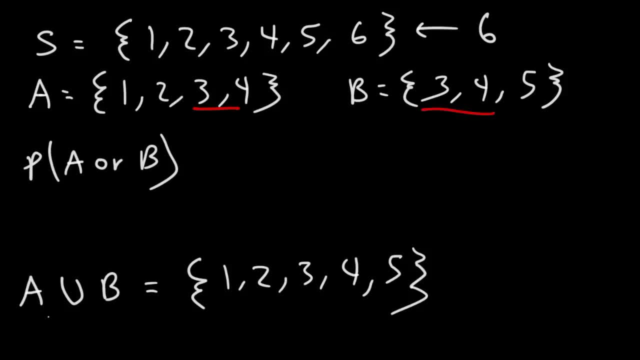 this will include everything except six. So there's five favorable outcomes that lead us to get an event A or B out of a total of six possible outcomes. So the probability is five over six, which as a decimal that's approximately 0.83.. 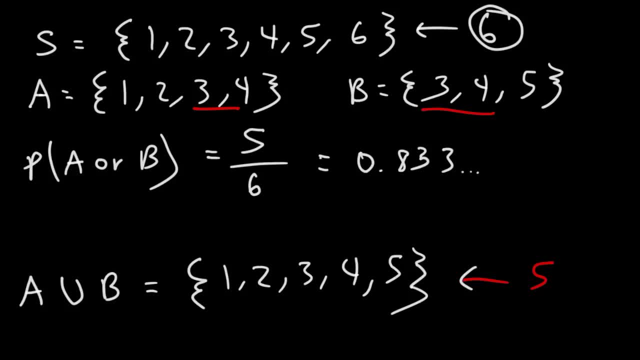 The three is repeated. So that's about 83.3% chance of getting A or B. Now what about the complement of A? What is the probability of getting a complementary event? Well, first we need to write the sample space of the complement of A. 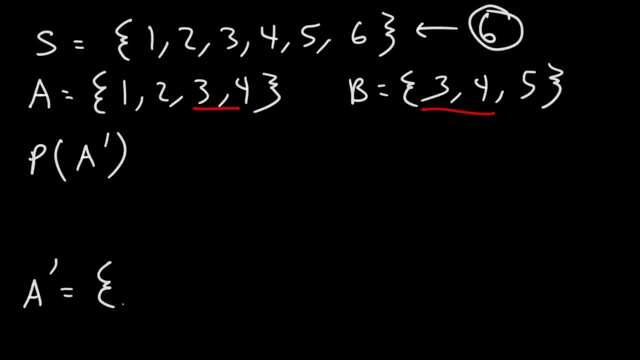 So this includes everything that is not A. So out of our sample space of one to six, A is one to four. So the other numbers that are not in A but still in our total sample space are the numbers five and six. 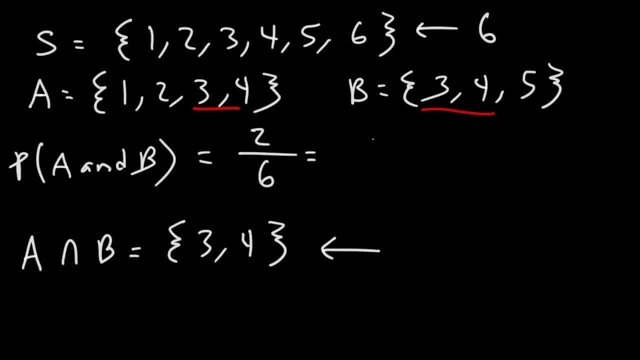 is going to be 2 over 6, which we can reduce. that 2 is 2 times 1.. 6 is 3 times 2. And so this becomes a probability of 1 over 3, which, as a decimal, that's 0.33 or 33%. That's the routed answer. Now what? 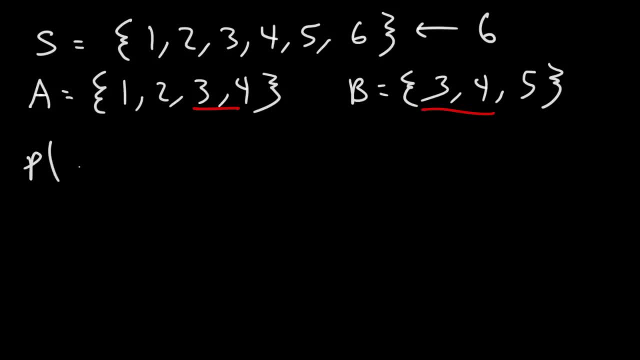 about the probability of event A or event B occurring. What's the answer to that question? Let's write the sample space of A or B, So this is going to be the union of these two events. So basically it's going to be all these numbers combined: Event A. 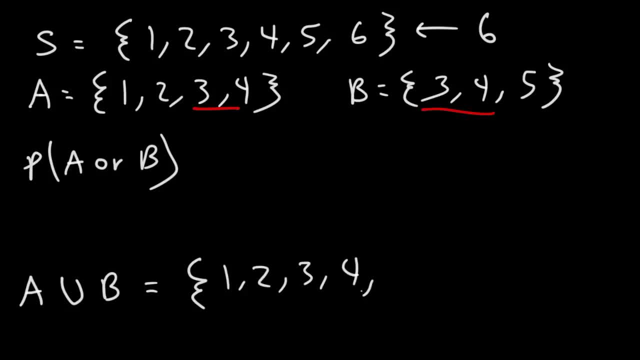 occurs any time we get a 1,, 2,, 3, or 4.. B occurs if we get a 3,, 4, or 5.. So this will include everything except 6.. So there's five favorable outcomes that lead us to get an event A or B out of a total of. 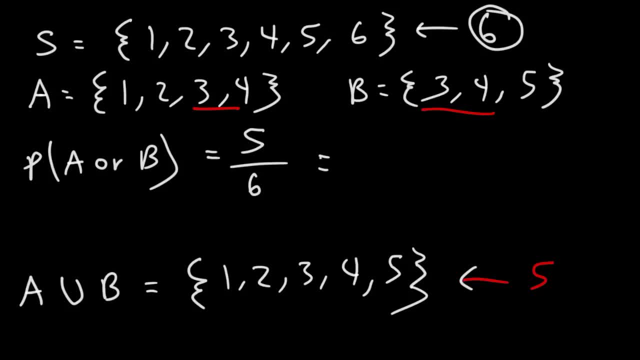 six possible outcomes. So the probability is five over six, which as a decimal that's approximately .83.. The three is repeated, So that's about 83.3% chance of getting A or B. Now what about the complement of A? 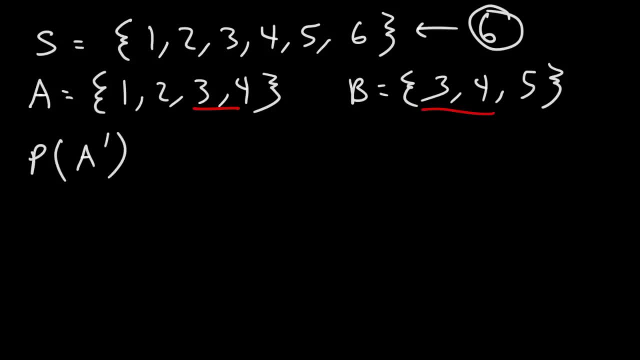 What is the probability of getting a complementary event? Well, first we need to write the sample space of the complement of A, So this includes everything that is not A. So out of our sample space of one to six, A is one to four. 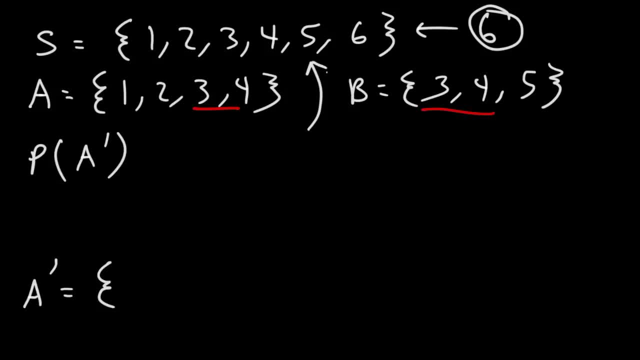 So the other numbers that are not in A but still in our total sample space are the numbers five and six. So the probability of getting the complement of A is going to be two. We have two favorable outcomes out of a total of six, which is going to be one over three. 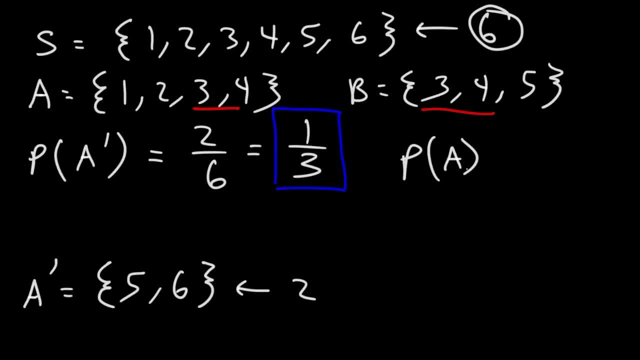 Now, what about the probability of getting A? Okay, So the probability of getting an event A or of event A occurring, what would you say? Now? there's four favorable outcomes that lead to event A out of six. So four over six reduces to two over three. 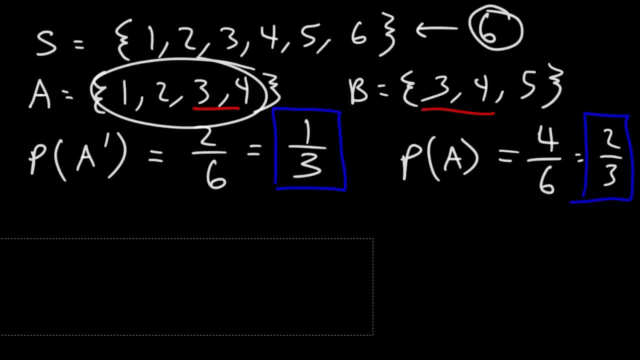 Now there's something that you want to take notice of. Notice that the probability of event A occurring plus the probability of the complement of event A occurring Adds up to one. P of A is two over three And P of the complement of A is one over three. 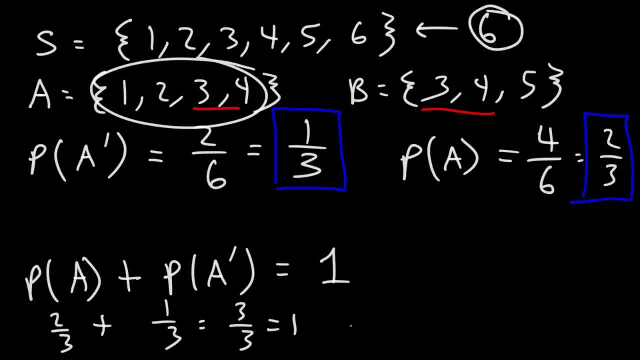 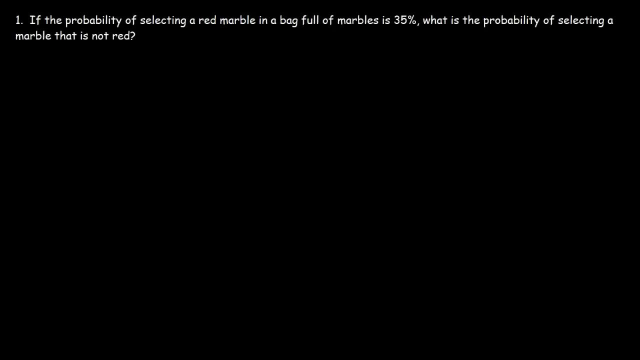 That is three over three, which is one. So this tells us that if we wish to calculate the probability of a complementary event, it's one minus the probability of that event occurring. Make sure you write this equation down, because it's going to be useful in the future. 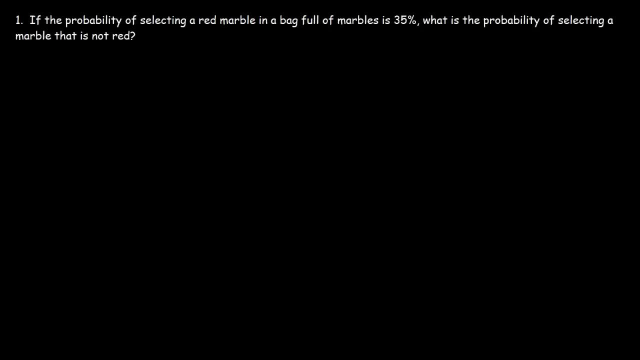 Let's work on this problem. If the probability of selecting a red marble in a bag full of marbles is 35%, what is the probability of selecting a marble that is not red? So the probability of getting a red marble, we're told, is 35%, which is 0.35.. 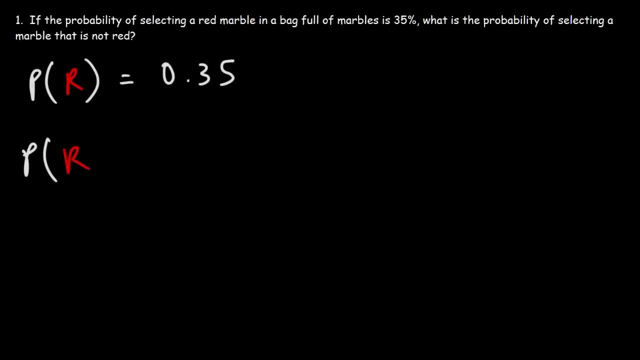 So what is the probability of getting a marble that is not red? So this proof: силU 드� angle: it's not red, It is negative. So what is the affinity value of R or the complementary of R, Based on the formula that we wrote before, it's going to be 1 MINUS. the probability of 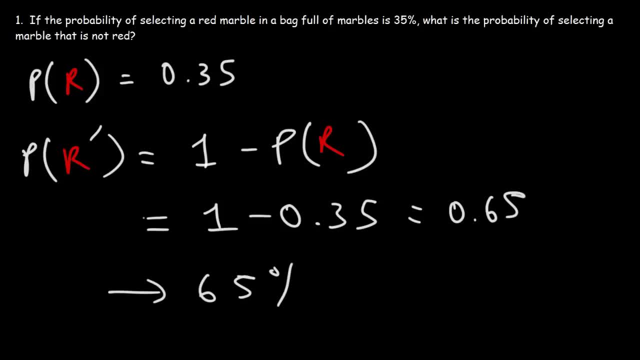 getting a red marble. So it's 1 MINUS 0.35.. Which is 0.65.. So there's a 65% chance of the getting a marble that is not red. Console sentence Subtitles by the Amaraorg community.